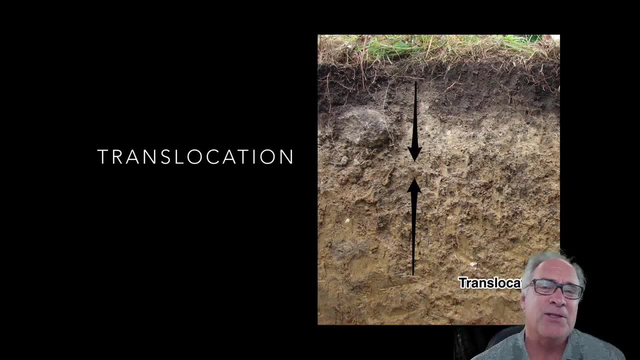 order. this is going on kind of in a cyclic manner, So it doesn't necessarily have to be in any particular order because it's going on from day to day. But translocation, and when we take a look at it, it's all about the transportation of materials from one part of the profile to 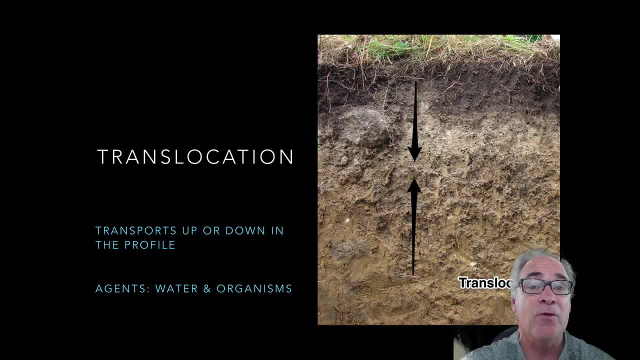 another. Mainly it's water and other organisms that move things around And when you've looked at some of the profiles you didn't see nice straight, even lines between one horizon to the next, primarily because it's not a perfect system per se and water and organisms move it. 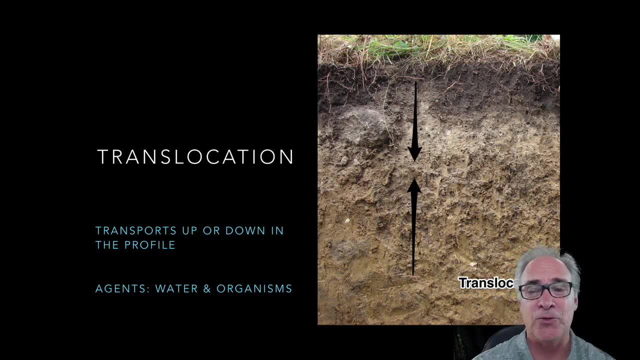 at different rates. So like, for instance, in this particular picture, you'll notice that white band, the E horizon. primarily the clay particles from the A layer find their way by water, via water, into that layer to create that other horizon that we recognize as the E horizon. 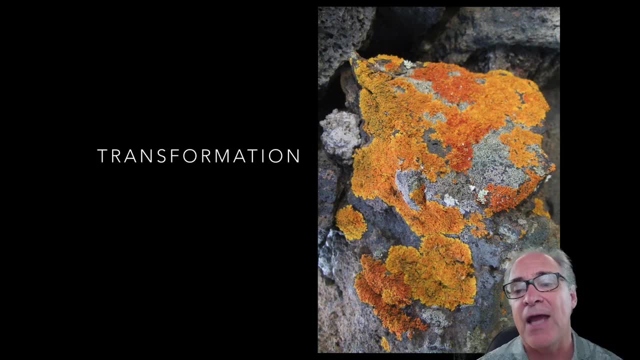 Alright. the last one is a transformation. Here's a rock that has some lichen on it and that lichen it produces some acids and other things that start slowly chipping away at the rock itself and breaks in smaller and smaller kinds of particles And at some point, this thing 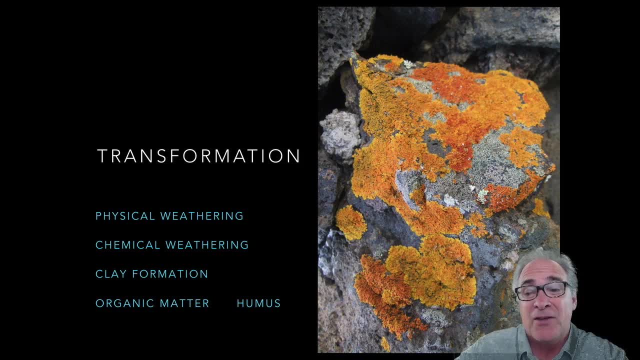 is going to be transferred or transformed, instead of this huge rock, into soil that plants and animals can thrive in. There's also, like I said before, because it's producing acids, a chemical as well as physical weathering that takes place And one of the things that eventually is going to 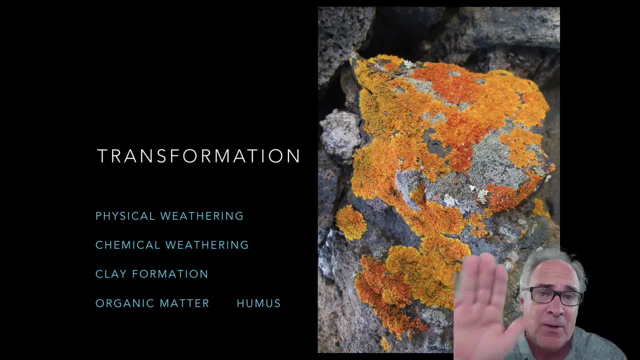 take place is some clay formation if you get them smaller and smaller particles and they keep eroding away. And then you've got a lot of other things that are going to take place and they're going to keep eroding away and weathering. you'll get to that Also. another great example is: 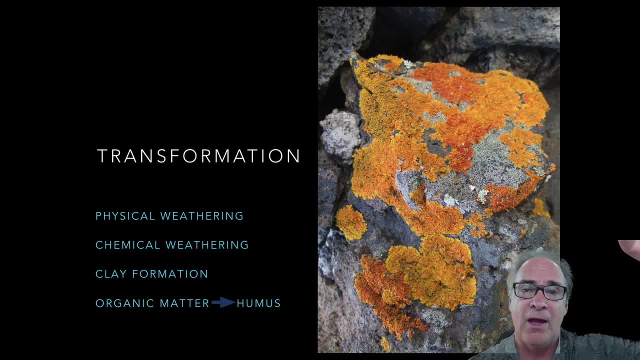 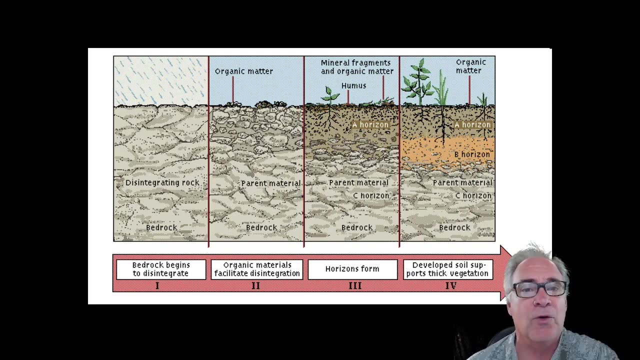 organic matter into humus. that happens between the O layer and also the A layer, And then, at the end of the day, what we have is a fully mature soil. We can start on the right-hand side- excuse me, on the left-hand side- and work our way across to the right-hand side. Each one of you should be able to.